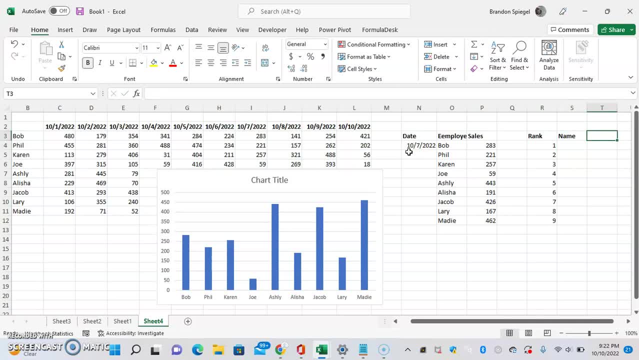 Then we are going to have a name column which you're going to fill in last, And now we're going to have a sales column, And here I'm just going to use the small function or the large function to be able to say: okay, with a large function, you know what's the first largest value. 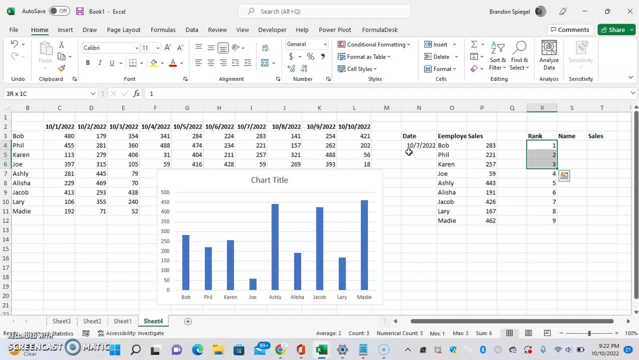 Then, what's the second largest value? What's the third largest value, Largest, and so on and so forth. With a small function. okay, what's the first smallest value? What's the second smallest value? What's the third smallest value? 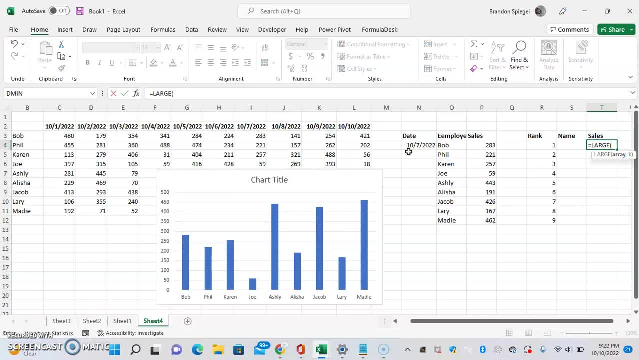 And so on and so forth. So let's just say: large function, Make something that is in descending order. The array is going to be the array they're going to try and define the values in. So here we're going to try to find these in the sales column. 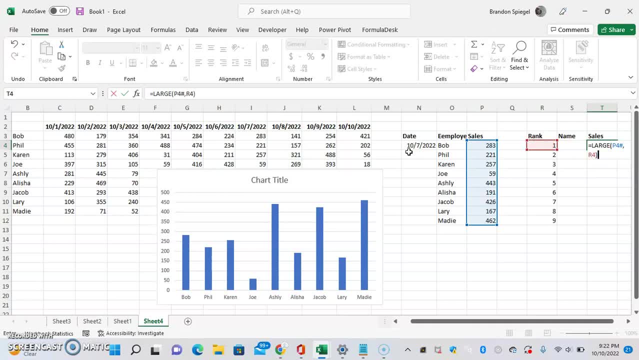 And then the k is going to suggest the rank. So that's the first Close parentheses. And then now we're going to lock this in real quick Function And F4. Because I'm on a laptop, or F4 if you're on a PC. 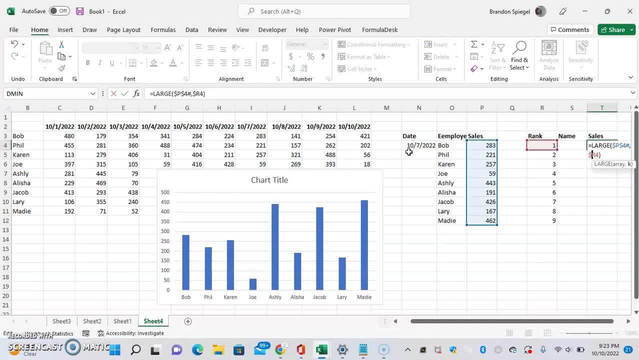 To lock that in. Sorry, not the R4.. That's going to be because I want that. to drag down Control C, Shift, Press down arrows, Control V And, as here you can see now it is in descending order. 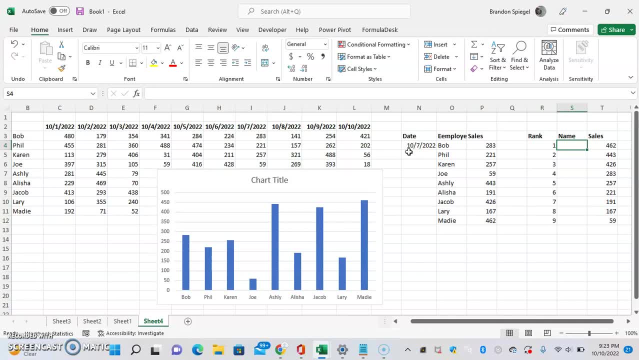 And then we can just do a lookup to do the name. You know, as you can see, the name is to the left of the lookup value in this instance. So I'm going to use the XLOOKUP function to do this Now. 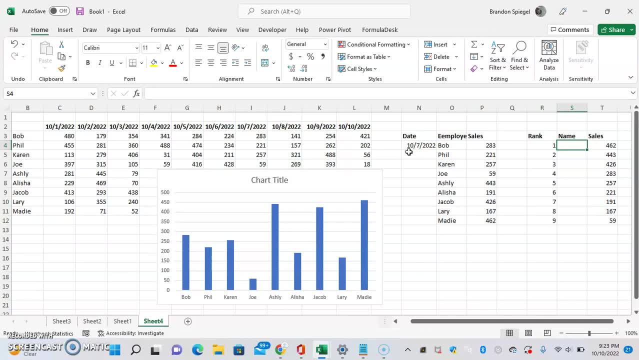 A quick note: the XLOOKUP function is came out in 2019.. If you're using Excel 2016,, you're going to have to do an index match Or rearrange your data to do VLOOKUP for this to work. 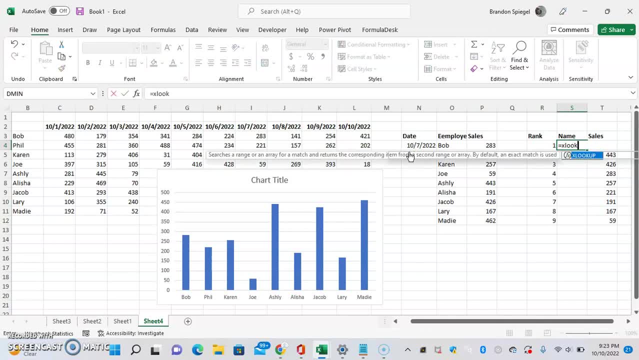 But this version of Excel XLOOKUP works. So XLOOKUP lookup value is just the sales value. Lookup array is where you're going to try to find the sales that. So I just say this right here, This right here. Then return array. 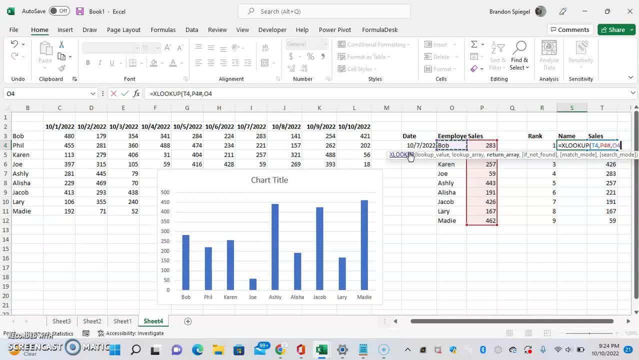 Is okay, We're going to. you know, what do you want to return? We want to return the names. We want to return the name that's based on sales, And then we're just going to. although there are arguments, are optional. 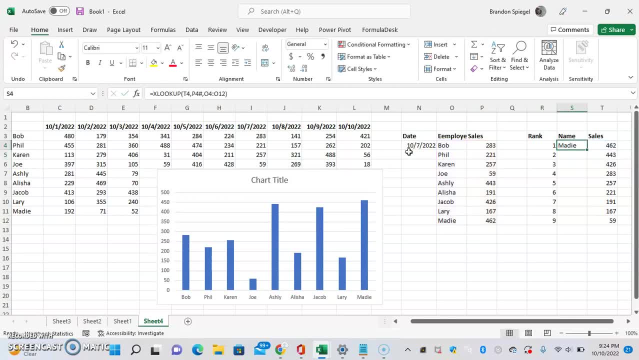 So you're going to just close it. Close parentheses. As you can see, Maddie had a sales associated with 462.. And we're going to lock this lock in these two ranges real quick with our dollar signs, Um, To make sure. 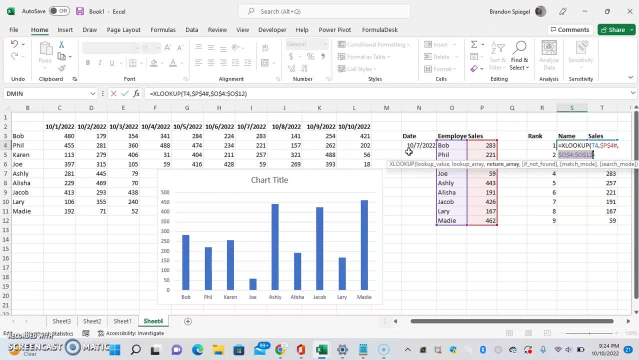 That you know, dollar signs in front of the rows in the column to make sure that it just isn't going to stay in place when you drag this down. Okay, And now you can see. it is an alphabetical order based on the name. 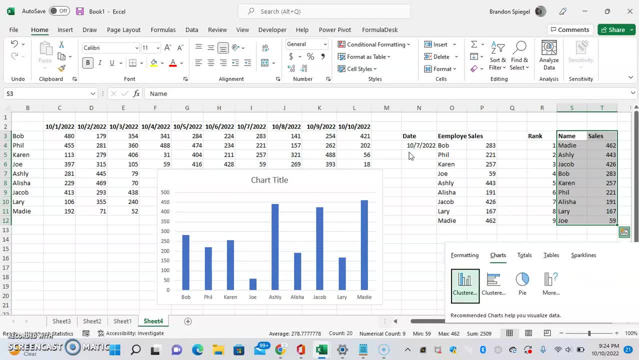 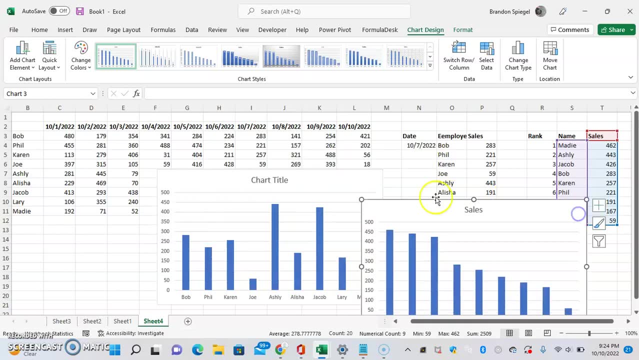 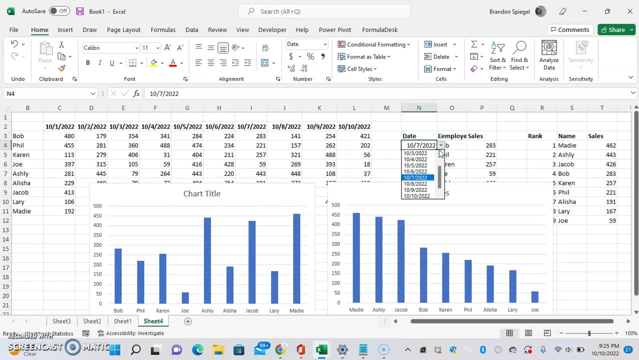 So now, when you highlight this press control Right arrow tab, You have a bar chart that is in descending order And looks much neater than the bar chart that we had Right here, And, as we can select, change the date, it is always in descending order, which, as you can see on days like this one right here, um, it makes much more sense, and the employee's name change as well. 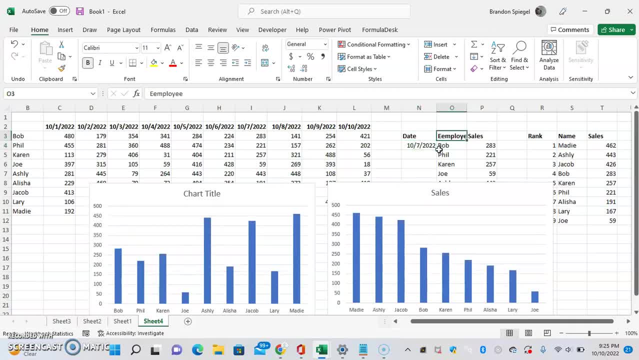 So on the first it's Bob with most sales, on the seventh is Maddie, And we can just kind of show what this would look like with a small function. You can change this for large to be small, So that way it is in descending order. 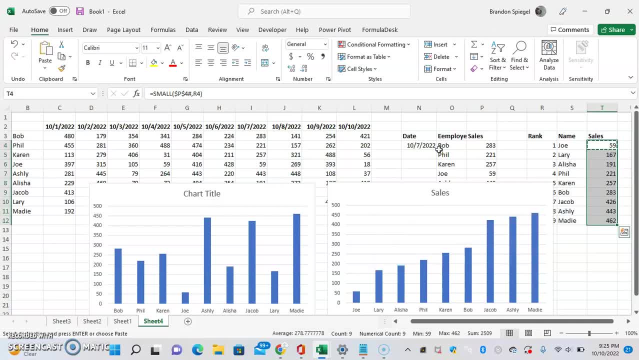 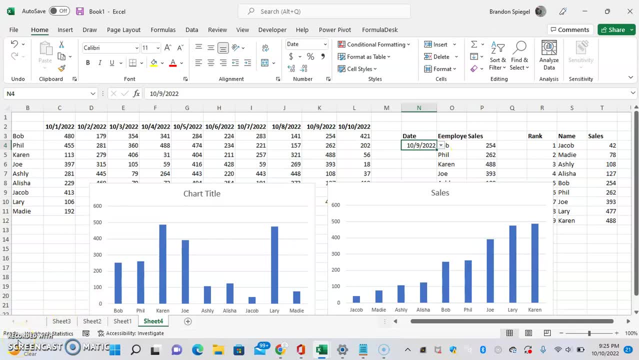 Or in ascending order, right. So now it's kind of flipped in with a small function. So there you have it, And real quickly to show you what it would look like with a lookup using index match instead of a X cup in case using the lower, your older version of Excel. 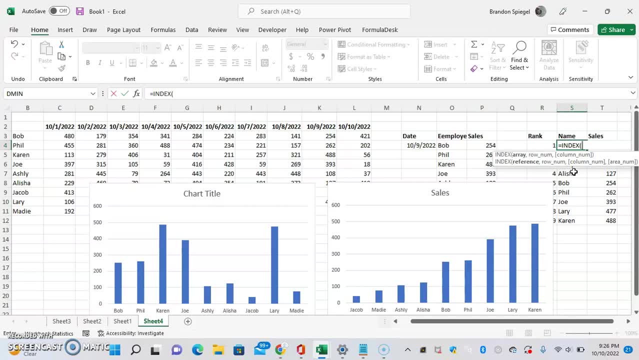 So that'd be index, open parentheses. Um, so index match is just basically a match function nested inside of an index function. So the array is okay. What do you want to be returned? Right, The equals index. first print is open. the array. 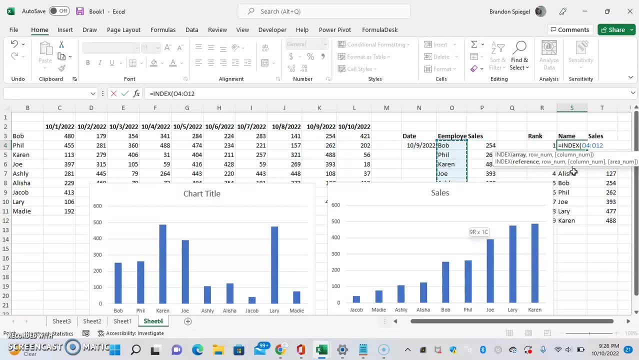 Okay, What do you return? Whoa, In this case, you want to return the name. So there's a name. Then the match function is going to be used to find the row number or column number that um returns. We're looking for there. 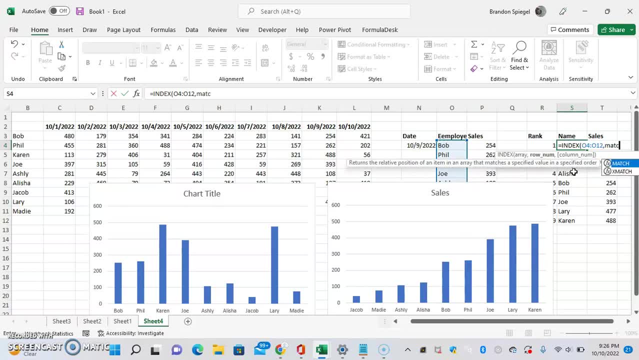 So match, not match. match. open parentheses. lookup value: Is it going to be the sales? lookup array is going to be the sales, right here. And the match type is optional, as you can tell by some brackets, but more often than not it's going to be zero for an exact match. 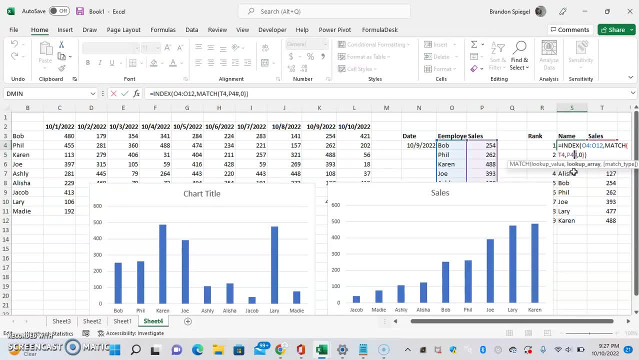 You might have to toy around. just that doesn't necessarily work the first time. One quick note: with this: um, right here again, newer version of Excel, um, the hashtag, um, so new Excel just kind of close to 65, just kind of, or isn't actually spill. 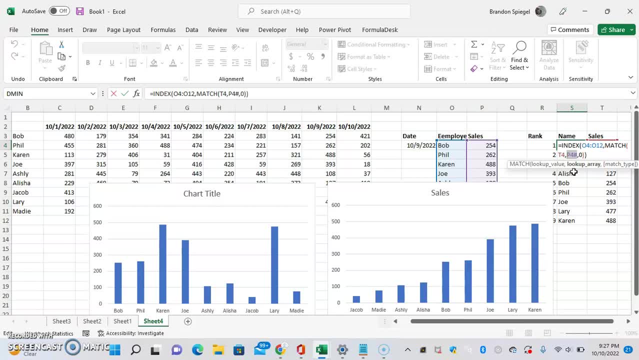 Um, just, which is why you see the, the hashtag. But just as a quick note. so function F4 to lock that in. function F4 to lock that in and then control C, shift, control down arrow, control V. um, just so you can see how you can get this to work on an older version of Excel with the index match. 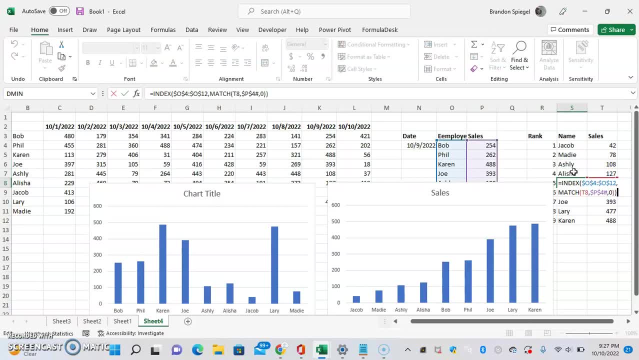 Um, if exec up doesn't work on yours, that's it. I hope you found this to be helpful to. uh, I hope you found this to be helpful, Um, and, if you did like, subscribe comment. thank you for watching. Have a great day. Have a great day. 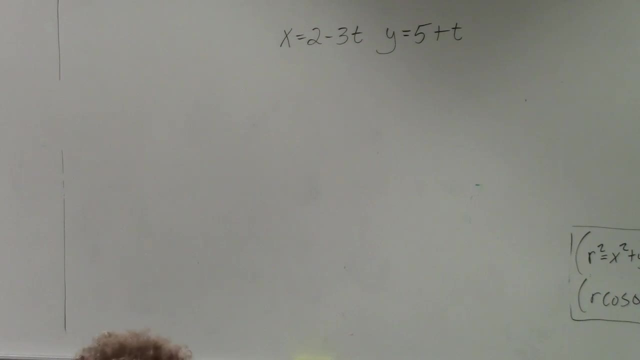 Where'd my cap go? Oh Yeah, usually my Algebra 2 classes would pick that up for me. I would have if it would have stopped, but it would have ran all the way under the deck. Alright, so in this example, what they're asking us to do is eliminate the parameter.